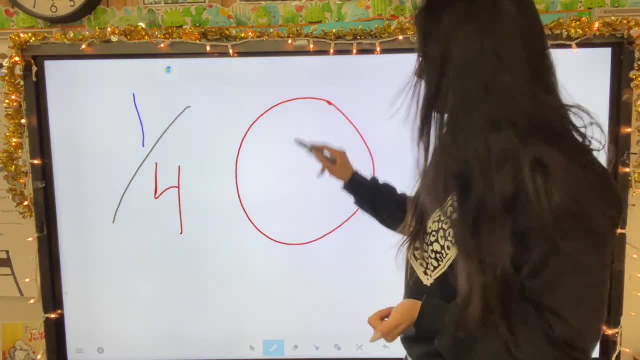 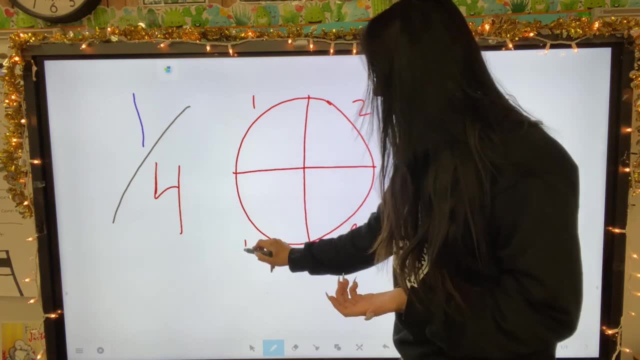 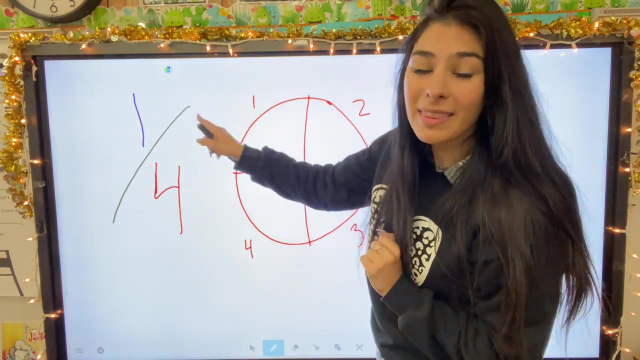 This one is kind of like a pizza or a pie That has four pieces: One, two, three and four. So here is my four, which shows the denominator, And now the numerator is one. That means one of these pieces is going to be shaded in. I'm going to eat one big slice of this pizza. 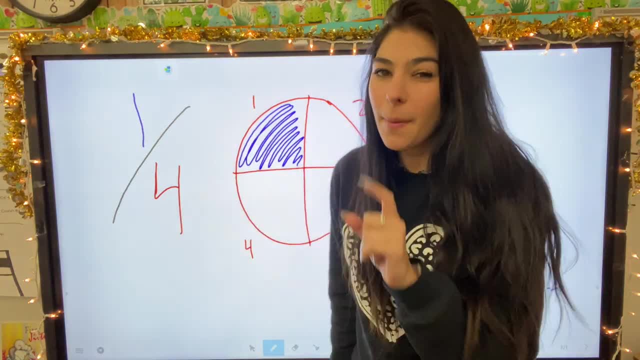 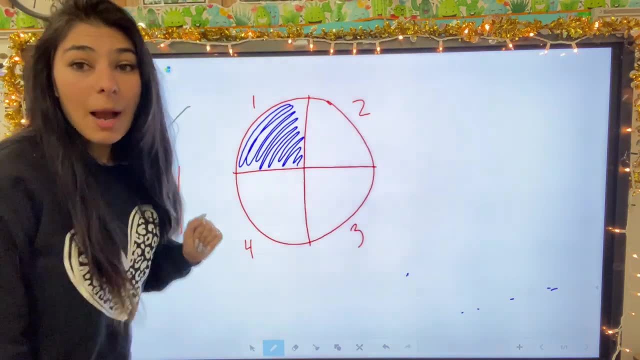 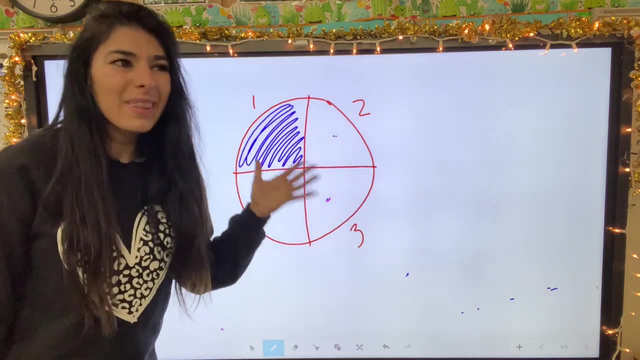 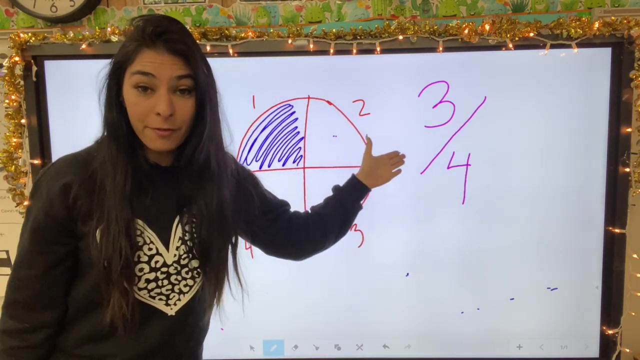 So now one fourth is shaded. But can I ask you a question: How many pieces are not shaded? Let's go over here. So I'm looking now at how many are not shaded in. I have one, two, three, So the unshaded pieces are three over four. So three fourths is. 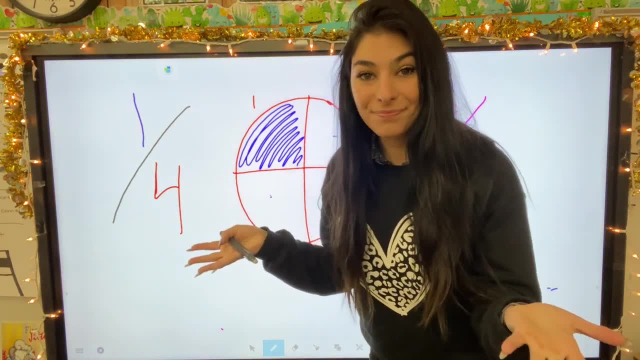 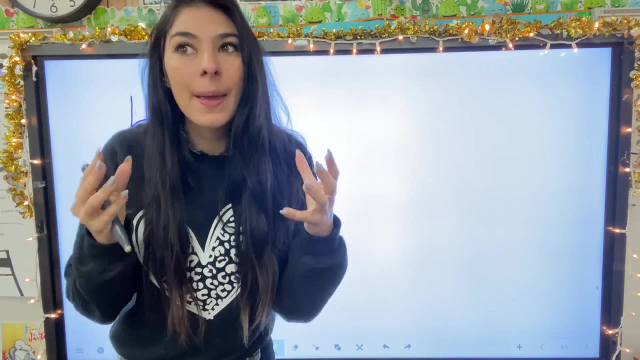 not shaded. One fourth is shaded. Let's do one more. Okay, I'm hiding this because before I show you this, I want to explain that fractions are So. another one is a total of four pieces of a whole object. Now I want to. 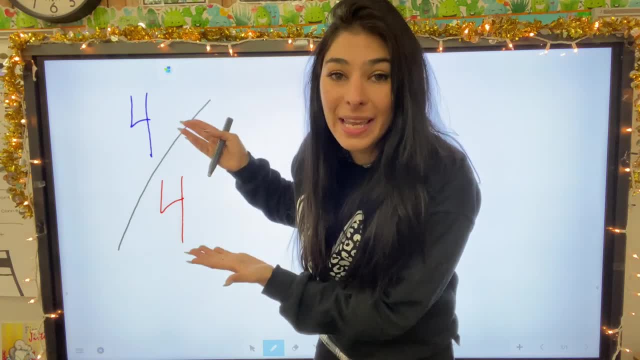 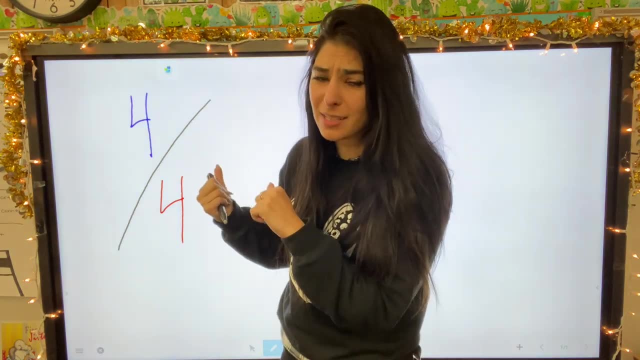 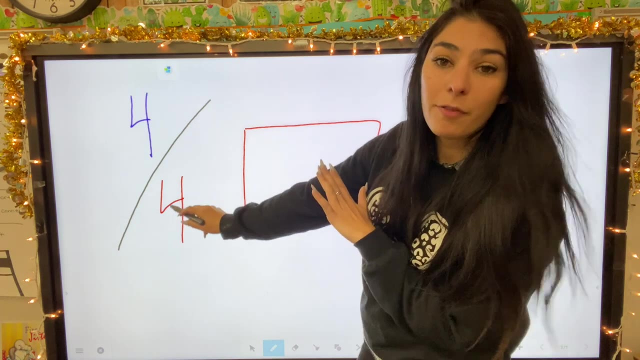 show you what happens when the denominator and the numerator are the same. So again, the denominator is the number that's down, that's the object and how many pieces it's cut into. weird. So I did a circle last time. This time I'm gonna do a rectangle. Now, when you are cutting these pieces into a fraction, all of the pieces have to be equal size. I can't do this. 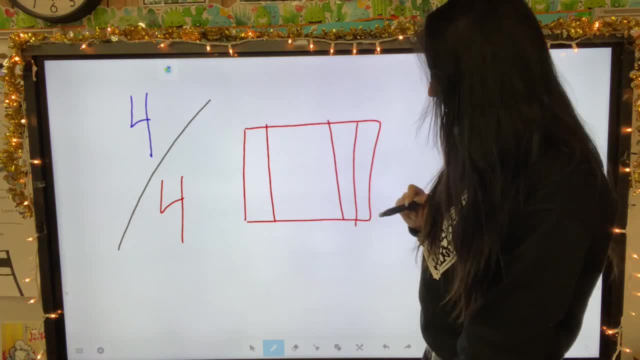 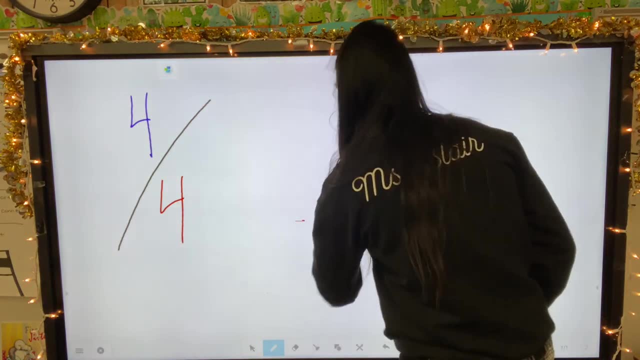 and then the other one, but I don't know which is the right shape. and then this: even though those are four pieces, they're not equal. therefore it is not a fraction. so I'm going to draw a square, I'm making it as even as I can. 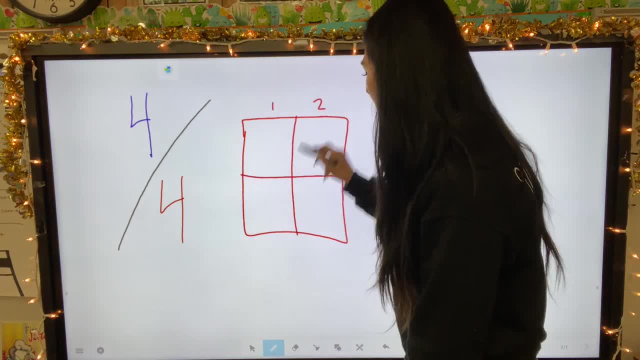 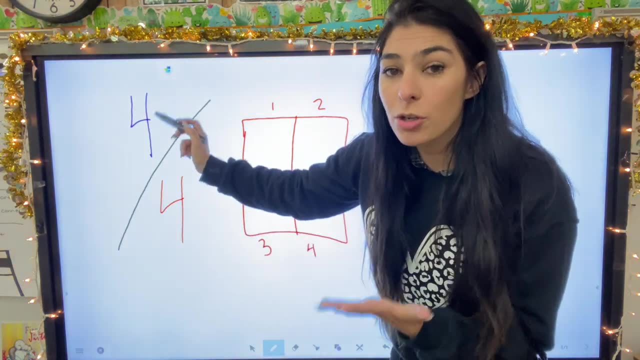 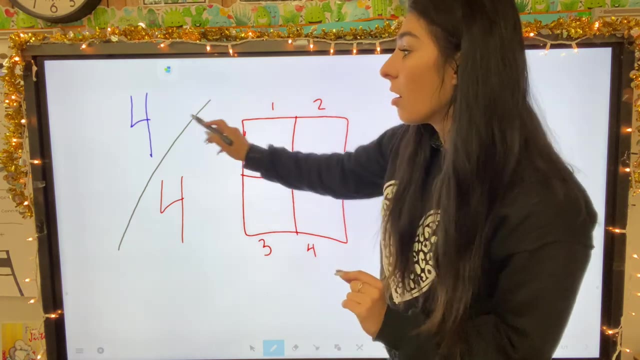 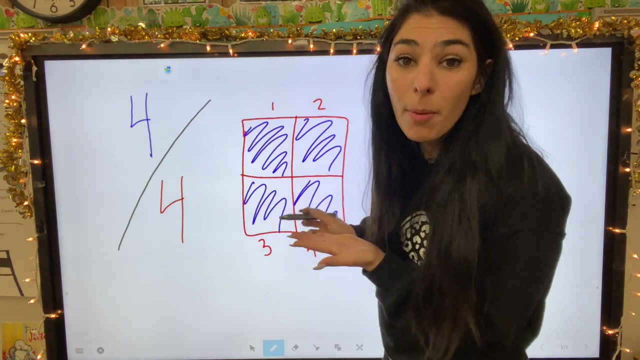 chop it into four pieces. I've chopped it into four pieces because my denominator is four, but now I'm gonna go to my numerator and my numerator is also four. so this is one object cut into four pieces. four of them are colored. how much of the object is shaded in? is there a piece of the object that shaded in or is?